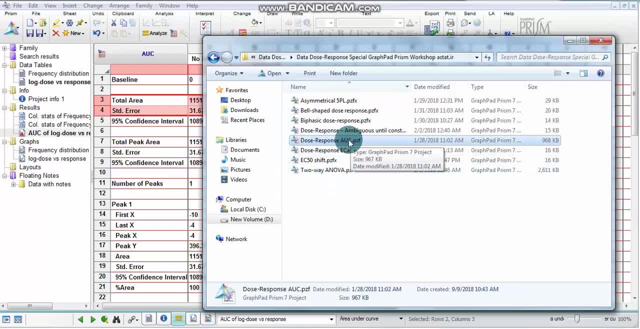 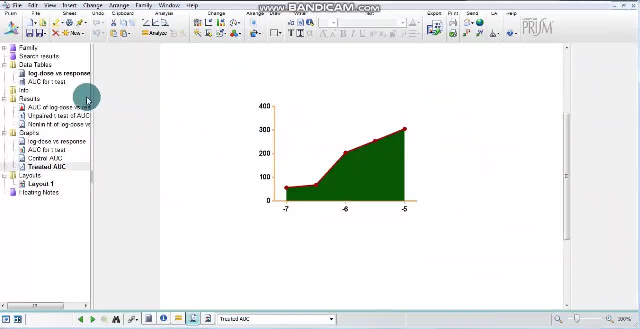 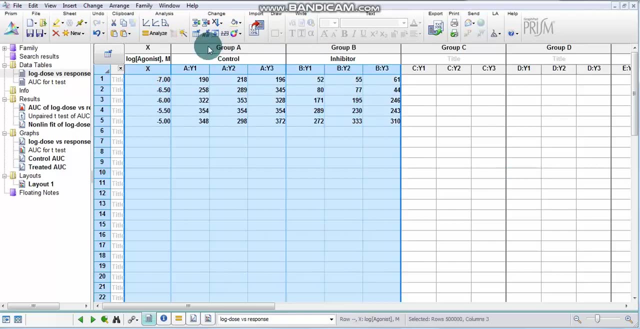 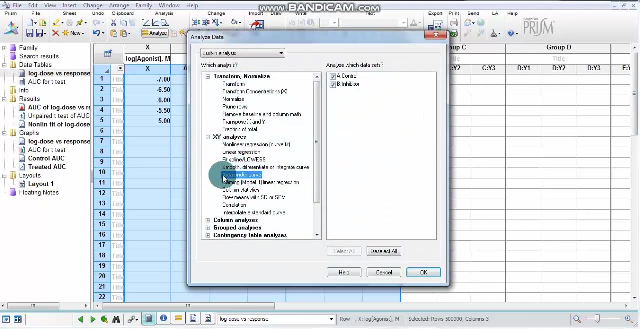 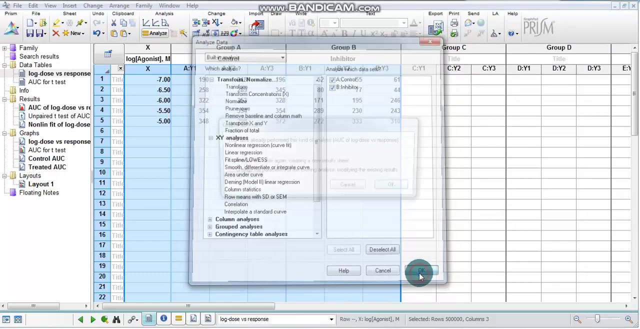 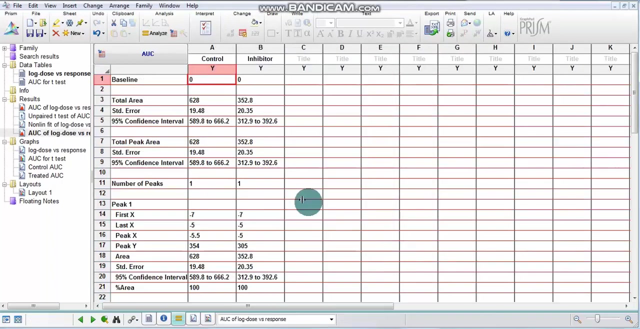 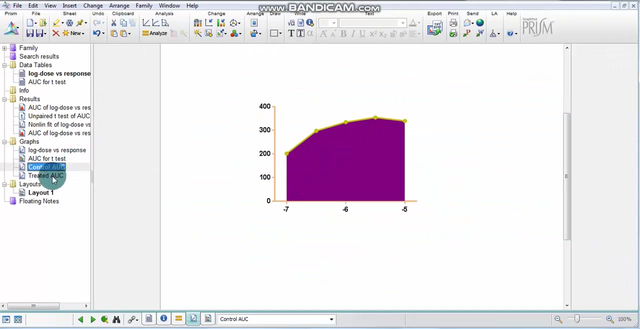 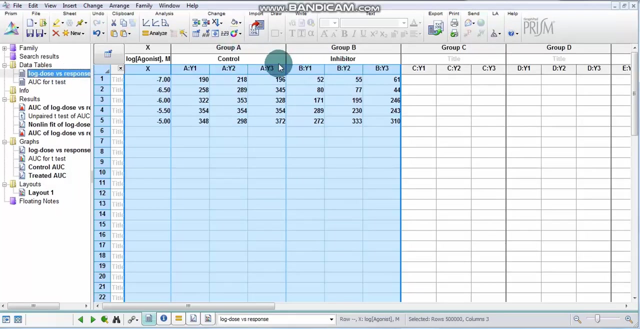 Thank you, Thank you, Thank you. 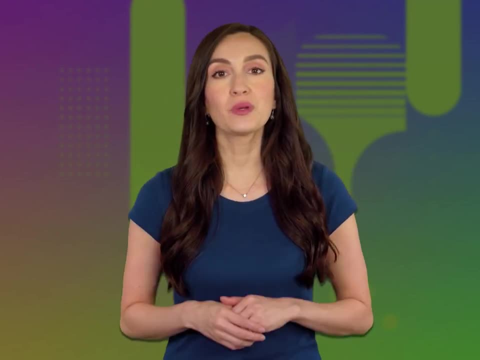 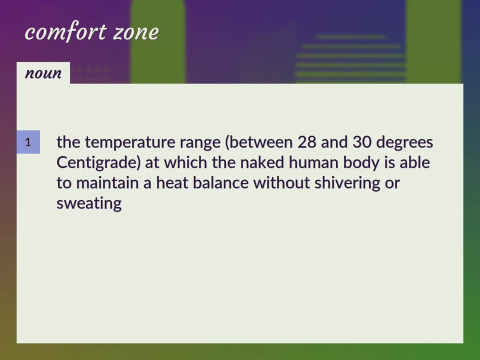 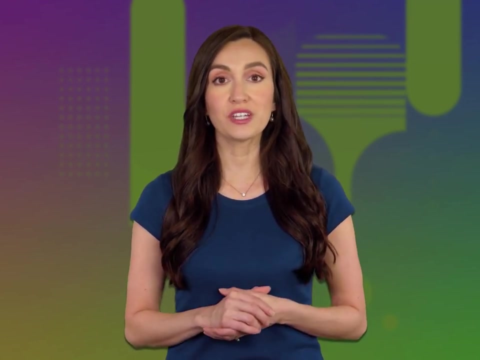 LanguageFoundation's video dictionary helping you achieve understanding The temperature range between 28 and 30 degrees centigrade at which the naked human body is able to maintain a heat balance without shivering or sweating. Become our student and get access to effective and free educational materials. 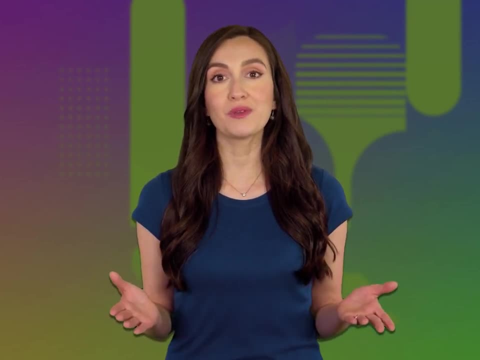 Subscribe to our channel to become a part of our growing community and to learn English effectively. 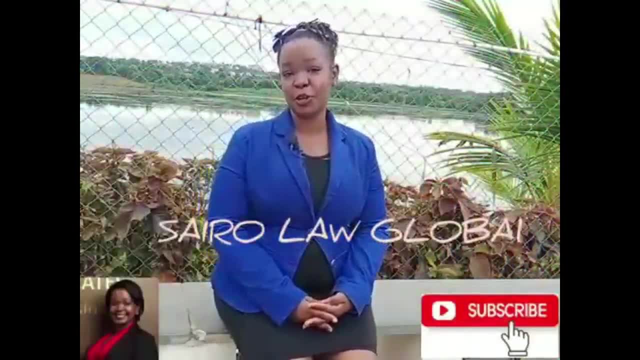 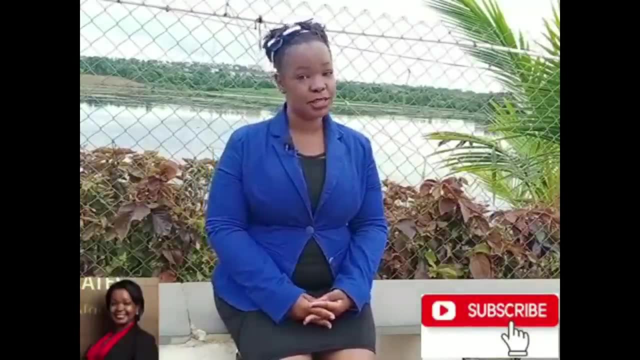 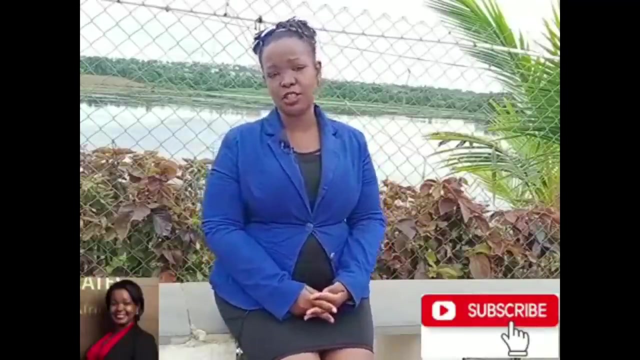 Hello and welcome to Legal Basics with Syrolo Global. My name is Sian. On this channel, we help you to demystify complicated legal concepts. Today, we are going to talk about a sale agreement. At whatever point in our lives, we may need to acquire or to sell property. Now it is very advisable that when you start this journey, whether as a buyer or a seller, you start it with a legal expert. 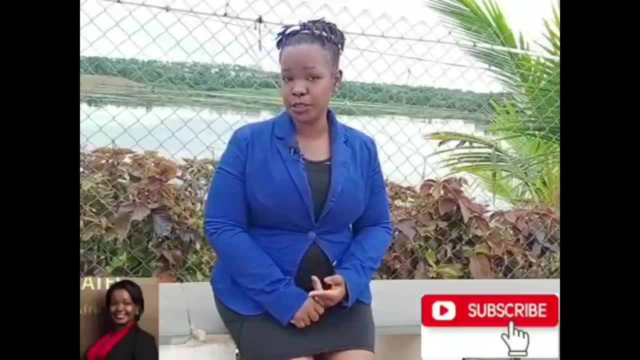 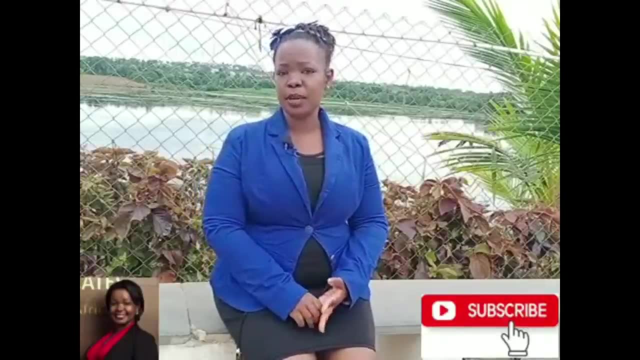 This ensures that you do not get duped by unscrupulous sellers and buyers. It also ensures that you do your correct due diligence. It also makes the process much easier and much faster and ensures that at the end of it, you have the correct documentation. 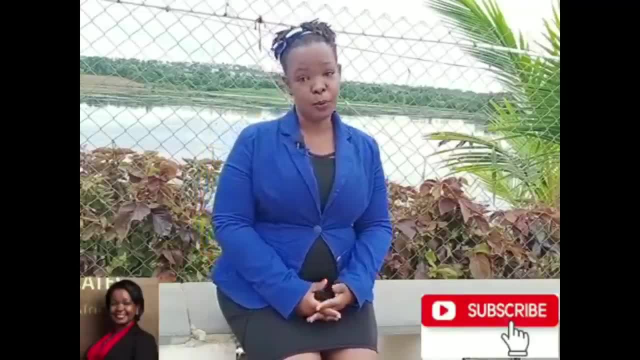 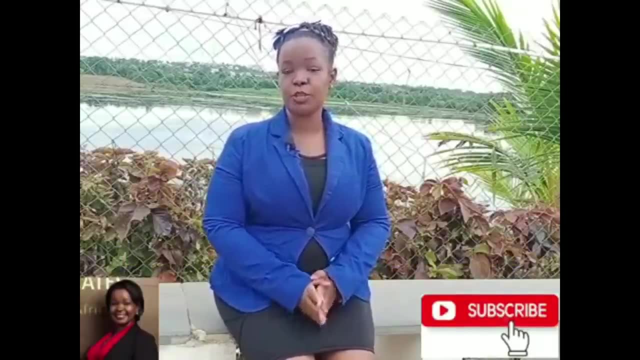 So what is it that you should look out for in a sale agreement? Number one: your sale agreement must be dated. If you and your seller are present on the day that you make your sale agreement, then in that case you must have a sale agreement.